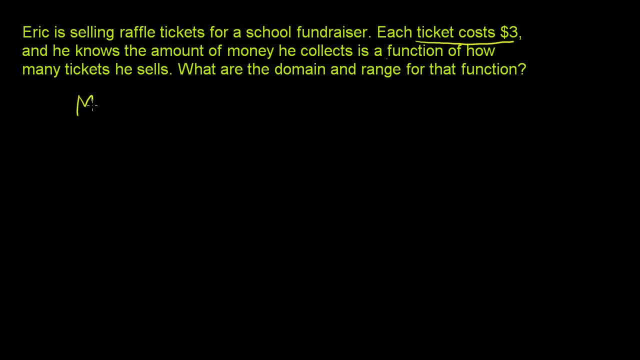 So I'll call that m. The function will be m, and it's a function of how many tickets he sells, So it's a function of t for tickets. So m, the amount of money he collects, is a function of the number of tickets he sells, and it's a pretty 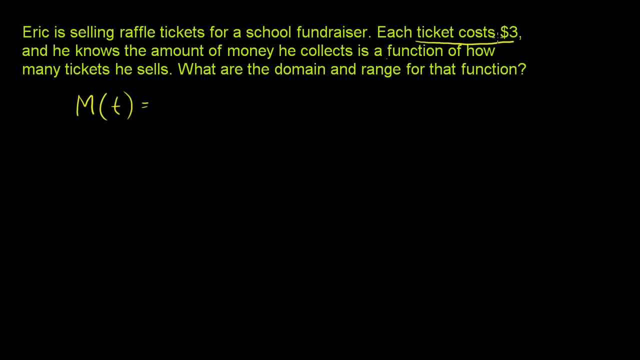 straightforward function. Every ticket costs $3.. He gets $3 for every ticket, So it's going to be 3 times t dollars or 3t dollars. That's how much money he collects. Now they ask us: what are the domain and? 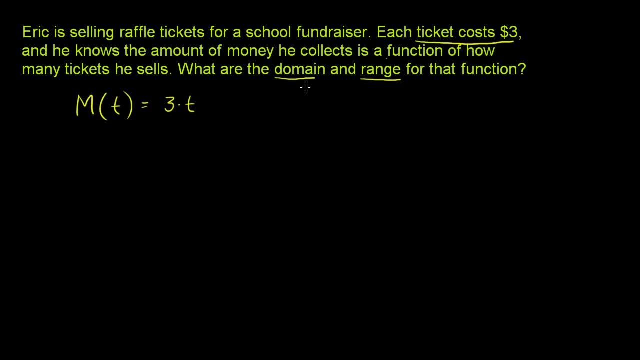 range for that function. It sounds all fancy and difficult, but just remember the domain. this just means: what can I input into the function? Can I input into the function? So another way to think about it is: what are the possible t's? 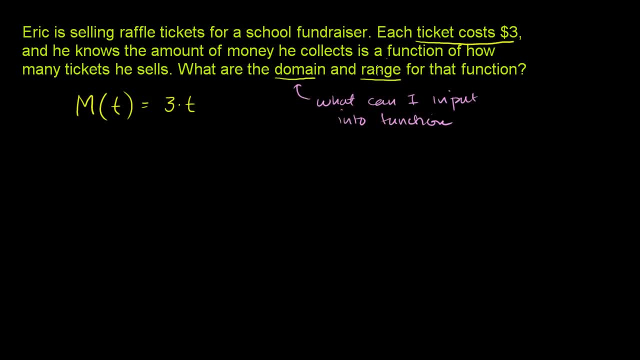 that can be input into this function. The range is: what are the possible values that the function can take on? So think about it. You might at first say, oh, I could put any t there. But think about the actual reality of what he's doing. 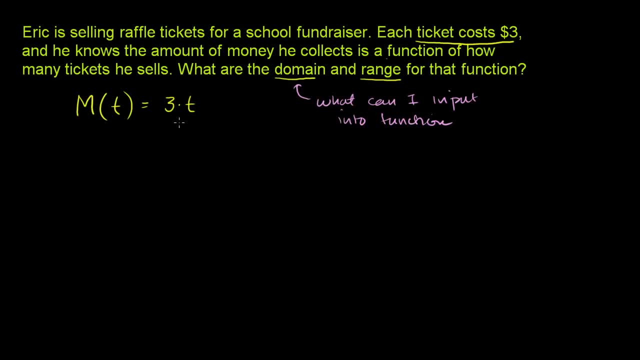 He is selling tickets And so we can't sell negatives. He might sell zero tickets and he might sell a gazillion tickets. I guess he could sell an infinite amount of tickets. At some point that becomes unrealistic. But he definitely can't sell negative tickets. 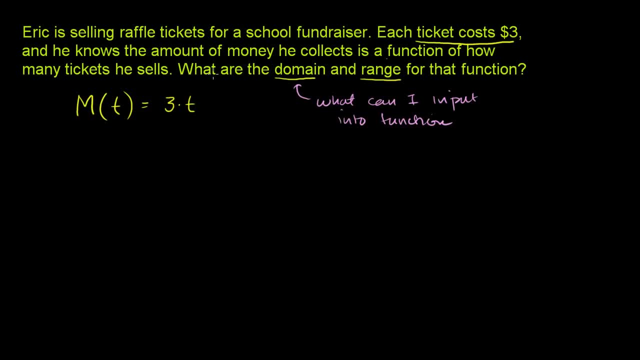 He also is not going to sell half of a ticket. Every ticket he sells is a whole number, It's an integer. So the domain for this function- the domain we could say t- has to be a non-negative integer. I think that covers what I just talked about. 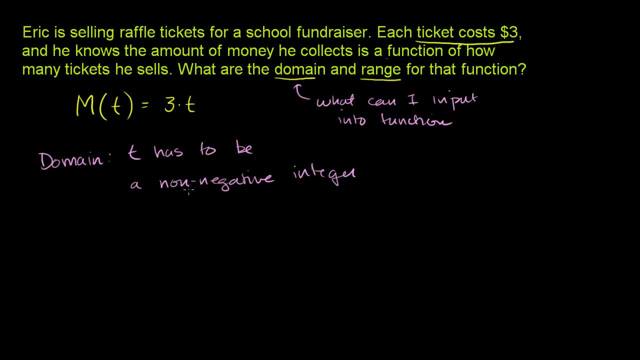 Non-negative Instead of saying pause because it could be zero. He might literally sell no tickets. He can't sell a negative one ticket or negative two, So it's anything that's non-negative And it has to be an integer. 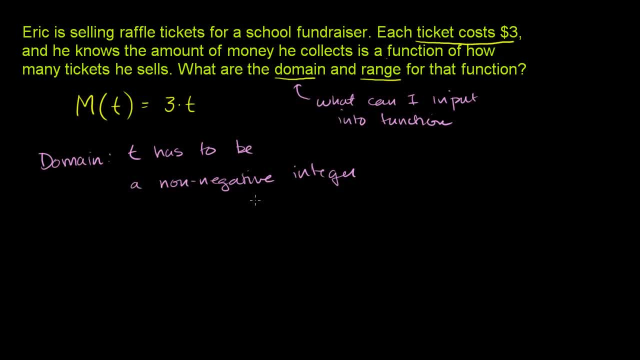 He can't sell half of a ticket. Well, it has to be an integer. So that's our domain, And let's think about what our range is. Our range is the possible values that we can take on If t is always going to be a non-negative integer.